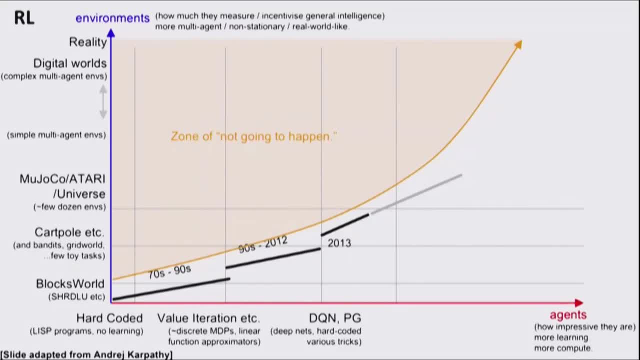 there for now and maybe they won't get there. So what I'm going to advocate for is that this is a way to solve not necessarily just the real world problems, but the real world problems, And that's a good idea- that to get there, to get past this possibility frontier. 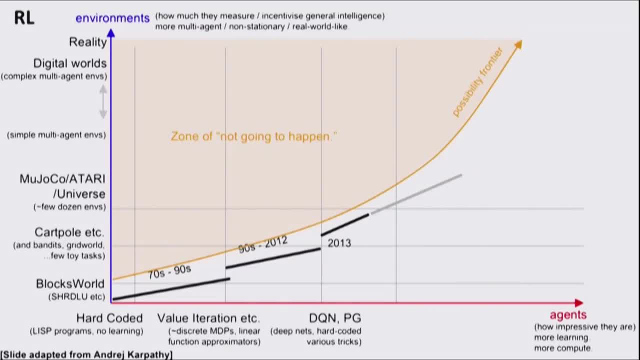 we actually need to somehow switch methods and do something that relies a lot more on data and compute and less on human ingenuity, And so what we'd have in the next generation of methods would be RL squared, let's say, a meta-learning RL method. 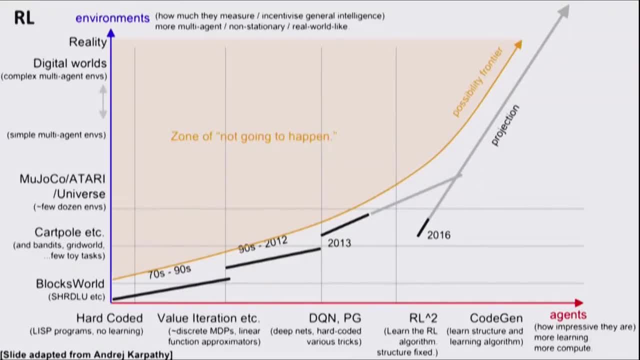 or even code generation, because often what's underneath what we do is code, And so I think to get to this real world type challenges and try to solve them, we'll need these kind of methods The further we move to the right on this axis. 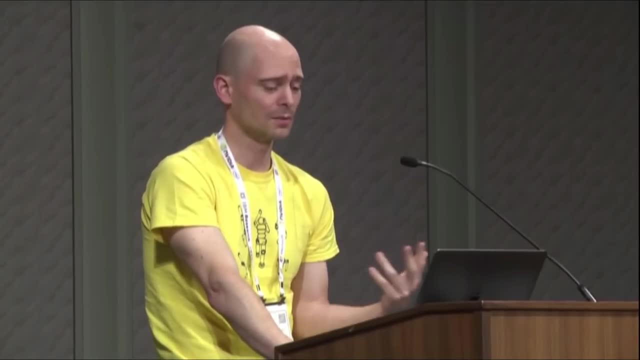 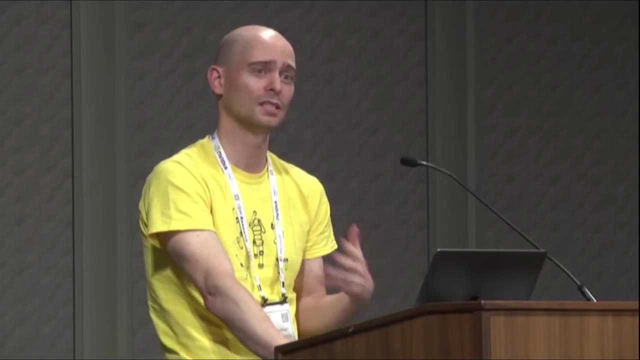 the more compute we need. So this will require that we have more compute than we have today, but we're also projecting that in the future we'll have a lot more compute than we have today. For example, many companies are building dedicated machine learning compute. 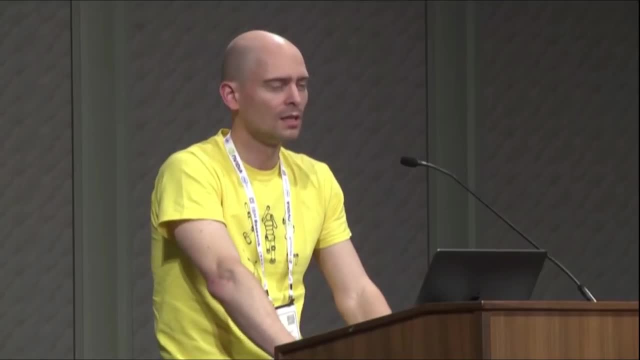 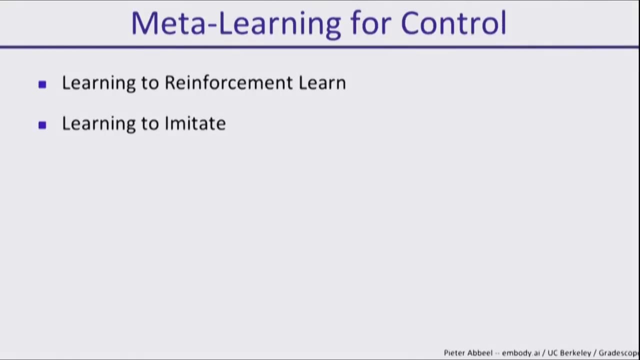 that we could leverage to move to the right on this axis. Of course there's a lot of meta-learning work already for optimization- Oriol summarized some of it- for classification, for generative models. Here I wanna focus on the control side of things. 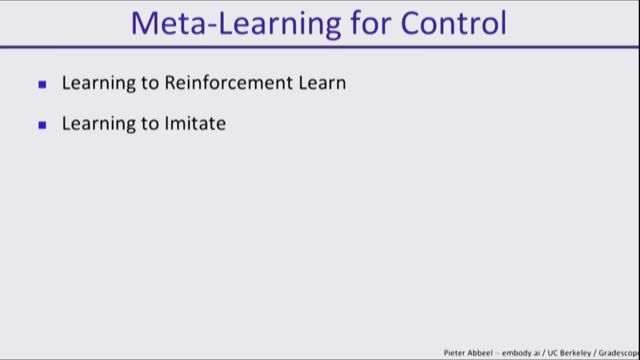 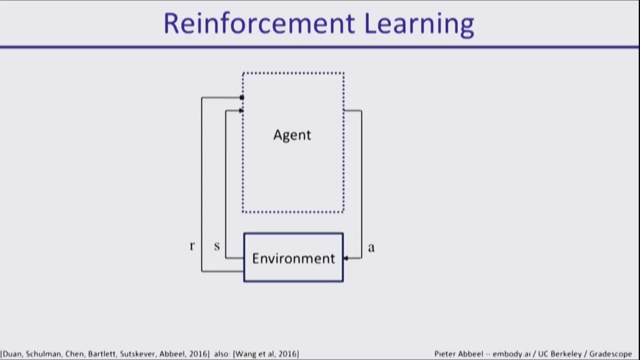 So one way to learn to control is reinforcement learning, where you learn from demonstrations, where you learn from your own trial and error. The other one is imitation learning, where you learn from demonstrations. So let's look at the reinforcement learning setting. We have an agent interacting with an environment. 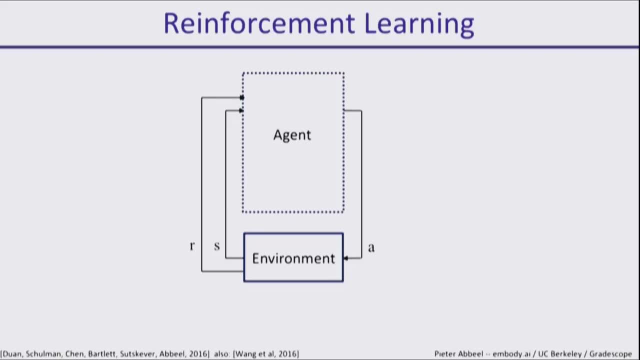 and hopefully it learns from that interaction with the environment to do better and better over time. Underneath usually we have a reinforced learning algorithm that updates a policy based on past interactions with the environment and hopefully over time this policy becomes good. When you have a new environment, let's say first environment A. 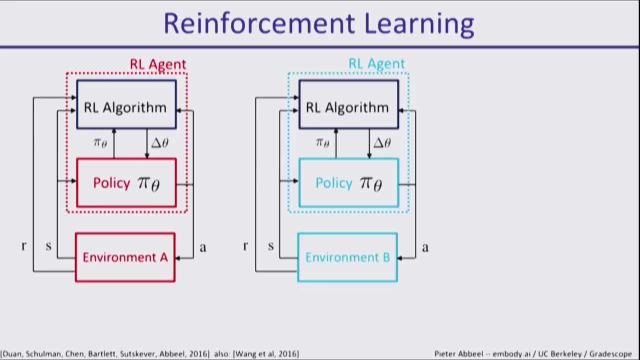 your algorithm will learn a policy for that environment. When you have a new environment, you can use the same code, the same reinforcement learning algorithm, but the policy will be relearned to now be tailored to environment B. Overall, what we see here is that 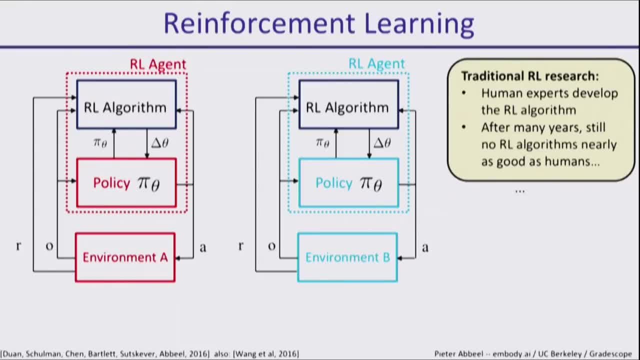 the agent consists of two parts: There's a reinforcement learning algorithm and a policy. Could also be a Q function. Human experts develop the reinforcement learning algorithm and then let the algorithm fine tune the policy. But even though we've spent at least 50 years now, 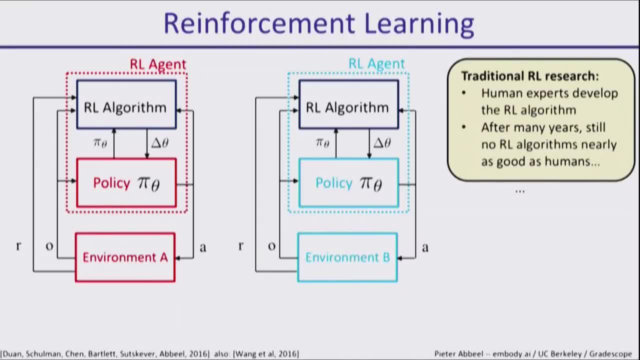 on designing reinforcement learning algorithms. we still don't have any algorithms that are as good as humans in terms of speed of learning, So maybe it's time to also let the other part be learned. Also learn the algorithm, So learn the entire agent, rather than only learn the policy. 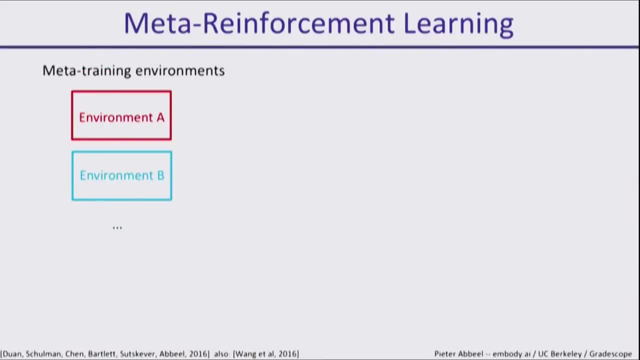 and design the algorithm by hand. So what would that look like? In meta reinforcement learning, what we do is we look at learning the reinforcement learning algorithms. So what that means is that we somehow are hoping that we can develop an algorithm that's learned. 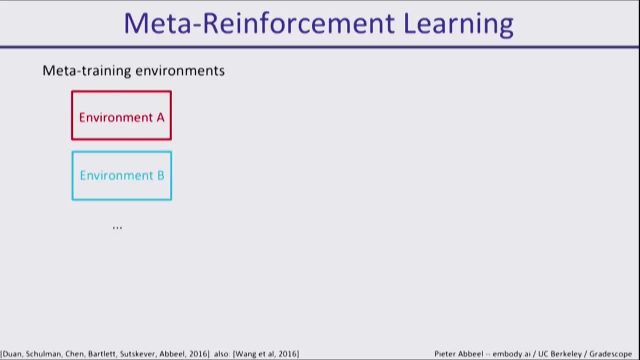 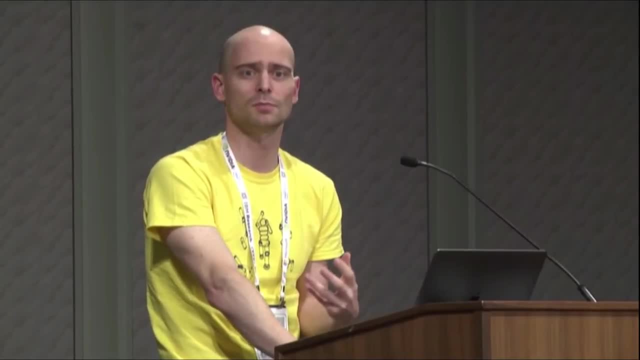 that's better than what we designed by hand, And the way that's going to play out. likely is that this algorithm is learned by seeing a lot of interactions with many environments And from that build up a prior over what the world tends to be like and code that inside the algorithm that now 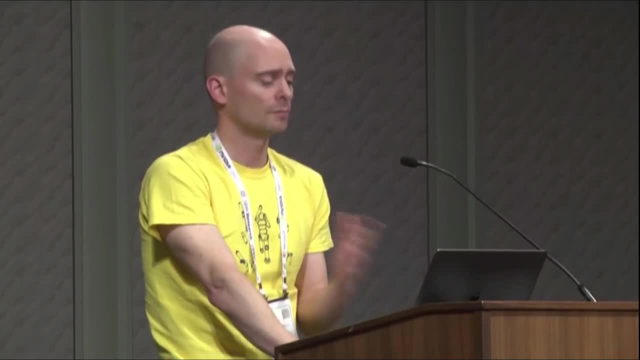 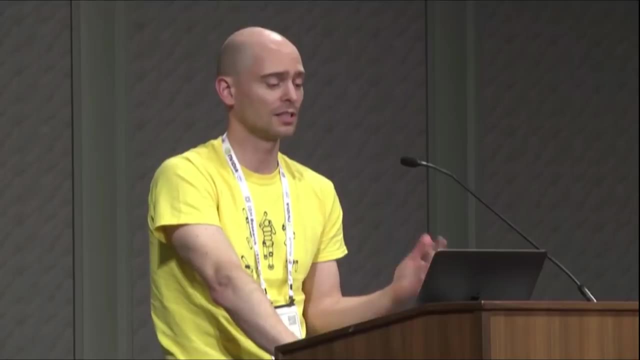 has a very strong prior allowing it to learn more quickly, So it might interact with environment A, B and so forth. And then somehow this meta RL box spits out a faster RL agent that is good at solving new environments very, very quickly. 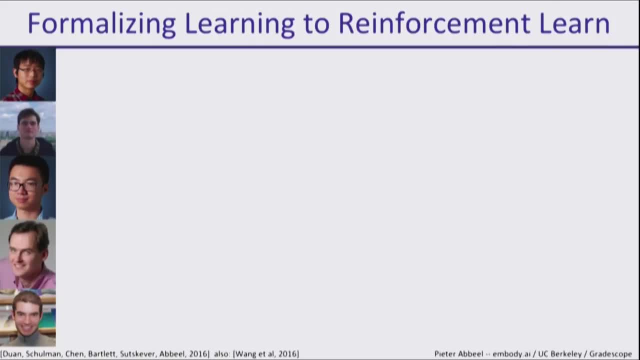 How can we formalize this? How can we formalize learning to reinforcement learning, This formalism that was published almost identically out of OpenAI and Berkeley, and then DeepMind. These are the two papers at the bottom. Here's the formulation: 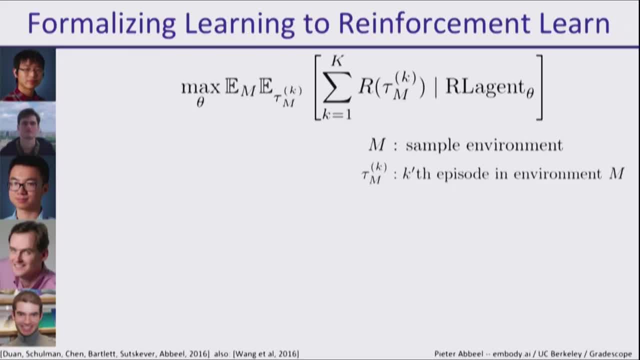 We'll try to find an agent, which means some parameter vector theta that parameterizes the agent. That could be code, It could be a neural net. whatever you think is a good representation of your agent. We want that parameter vector theta to be such. 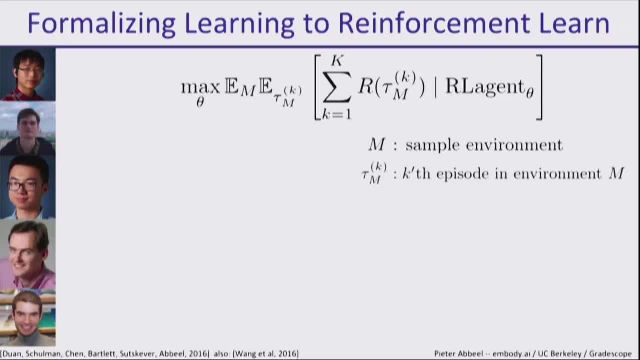 that if you sample an environment at random and then sample trajectories executed by that agent in the environment, That somehow that agent collects a lot of reward. Now keep in mind: this agent is not just a policy. It's allowed to adapt over time. 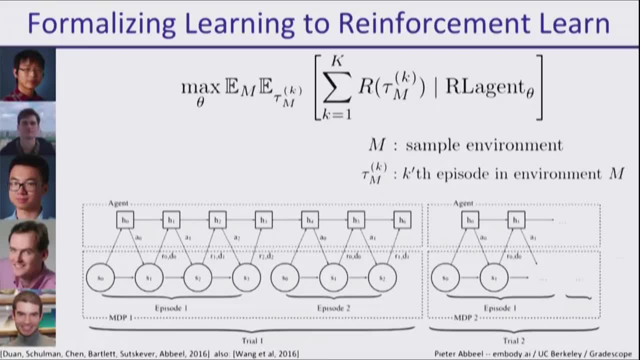 So it's going to be dropped in an environment, let's say, two times Over those two episodes, hopefully- has adapted, learned to do well in that environment and then it gets moved to a new environment And we're going to train it hopefully. 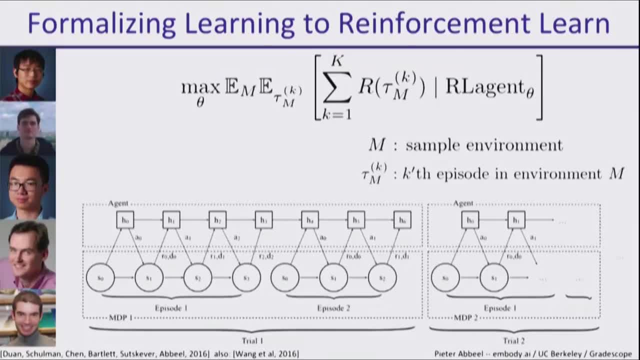 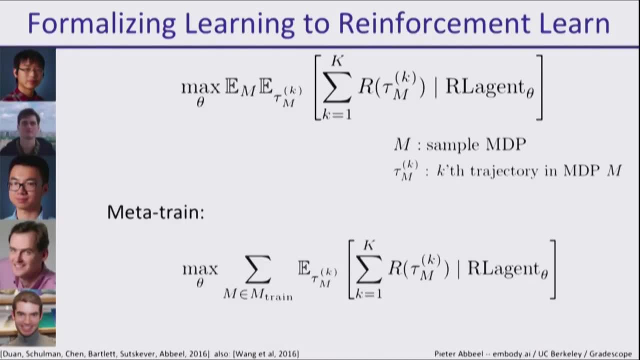 to be good at collecting reward in just capital K episodes in a single new environment. it's never seen before. So we need to make some choices for what we put underneath. So here's our training objective: We need to choose What this agent is going to be. 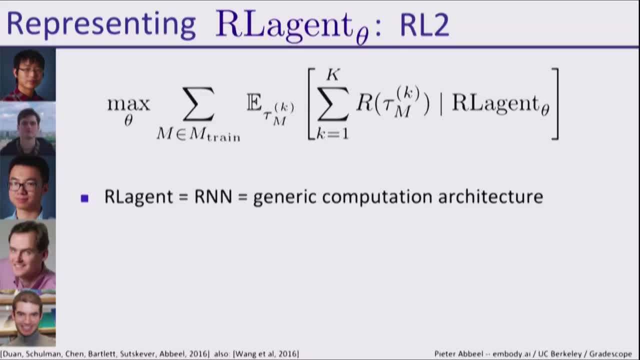 One thing we could put underneath is a RNN. The beauty of putting an RNN underneath is it's very generic. It can encode any algorithm. It can encode prior about environments and so forth. If you look a little more deeply, the weights in the RNN would correspond. 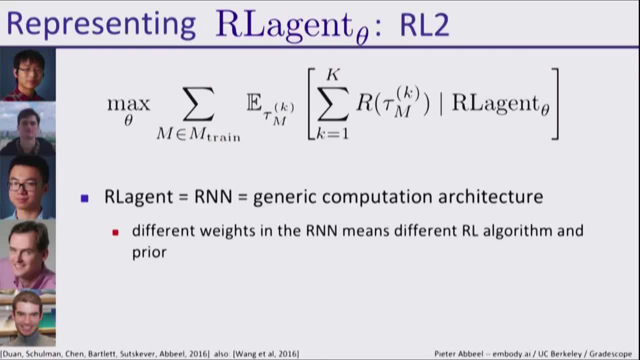 to both the reinforcement learning algorithm and the prior over environments somehow encoded in there. And then the different activations that the agent has over time would correspond to it adapting its policy as it's acting in a new environment. The meta training objective at the top. 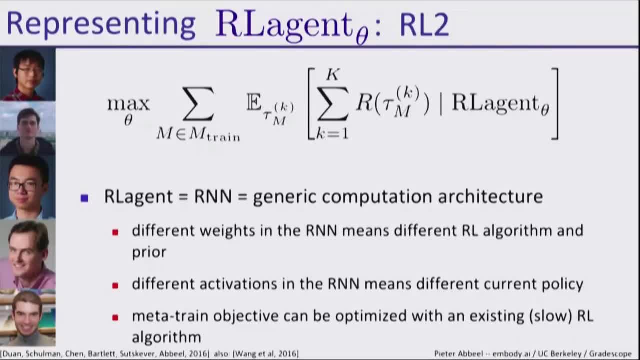 can be optimized for with standard reinforcement learning. So what we do is we bootstrap off of standard reinforcement learning algorithms, let's say PPO, TRPO, A3C and so forth- whatever is your favorite one. use that to optimize this objective. 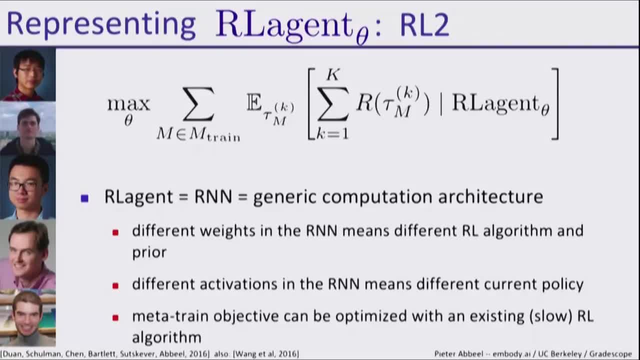 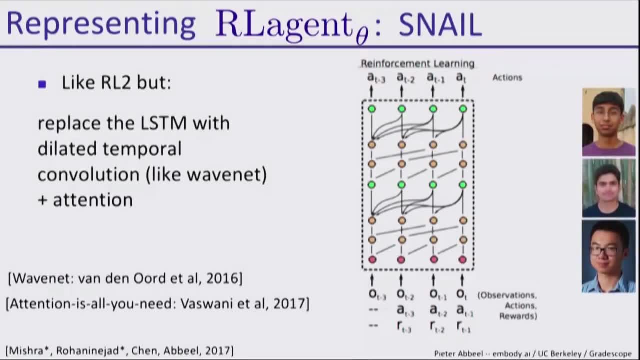 And the consequence would be a recurrent neural net. that itself is an agent that has embedded in it reinforcement learning algorithms that are faster Don't have to put an RNN underneath it necessarily. You can put something else, for example a WaveNet-like architecture. 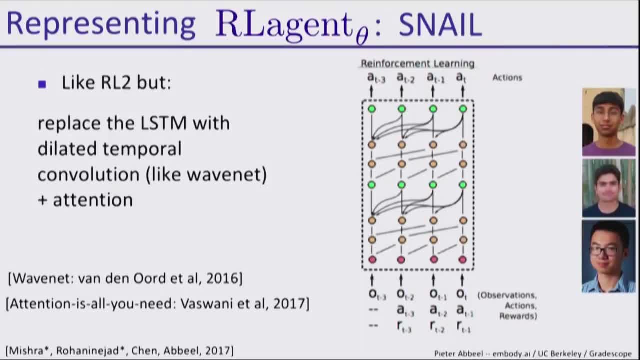 So dilate the temporal convolutions, but then maybe with attention also, so you can see more detail from the past than a WaveNet would allow you to see. You can use the exact same objective, just a different architecture for the agent underneath that's being trained. 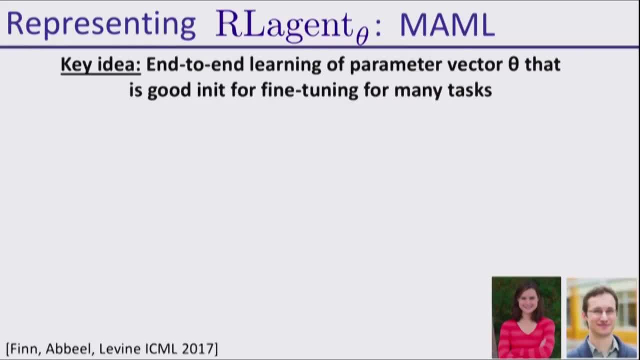 Or you can do yet something else. You might say: well, we know gradient descent is pretty effective, Let's stick with gradient descent And let's just see if we can pre-train an agent such that it's ready for fine tuning when it's. 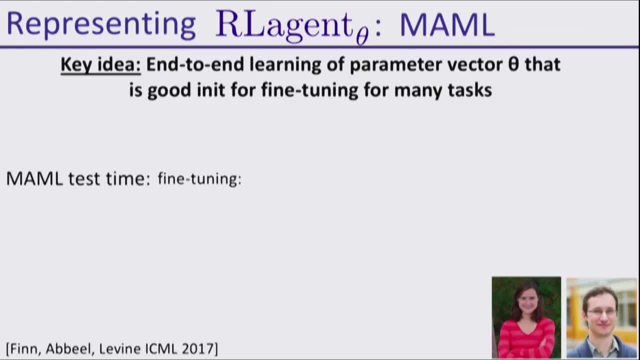 faced with a new environment. How would we set that up? This is called MAML. At test time, You're going to be fine tuning. So at test time you start with some pre-trained parameters, You get some new data, compute a gradient, do an update. 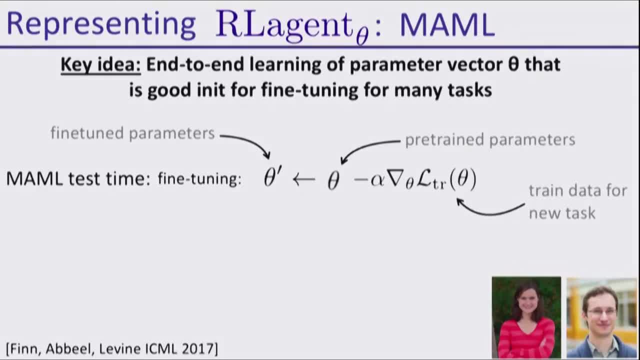 get a fine-tuned parameter vector And the hope is that this fine-tuned parameter vector is good at solving the task. How do you train for this? You can train this end-to-end. You can at training time. this is now meta-training time. 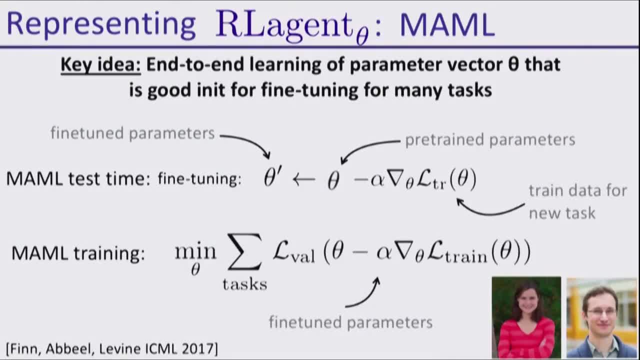 you can set up a set of tasks. You try to find a parameter vector, theta, that is such that if you sample a task and then take a gradient step on the training data from that task, that you do well on the validation data of that task. 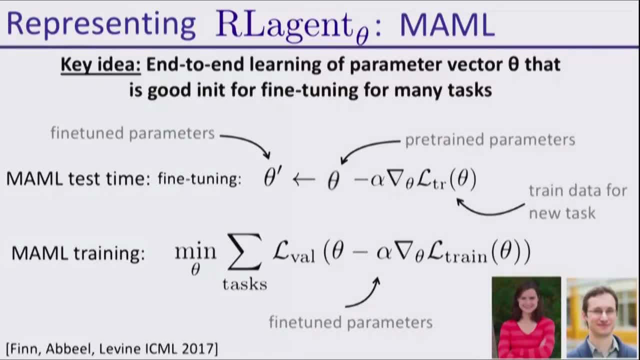 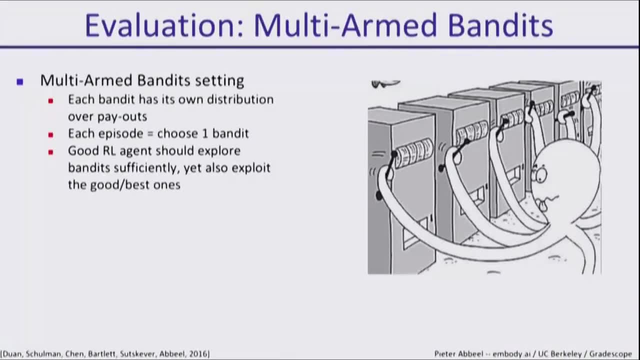 with just one gradient step. If you find a parameter vector- theta- that does this, then that's a really good, pre-trained parameter vector that you can use to solve many tasks in the future. Once you have any of these architectures, it's interesting to start looking at how well can they? 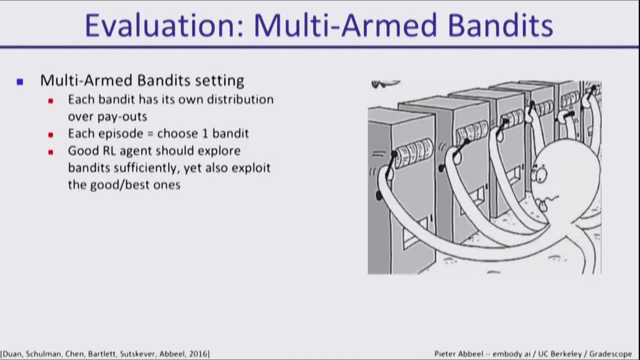 solve problems that humans have already solved. For example, band net problems, which are canonical reinforcement learning test problems, where you choose at any given time a band net to play. That band net has a probability of payoff, but you don't know ahead of time what the probability of payoff. 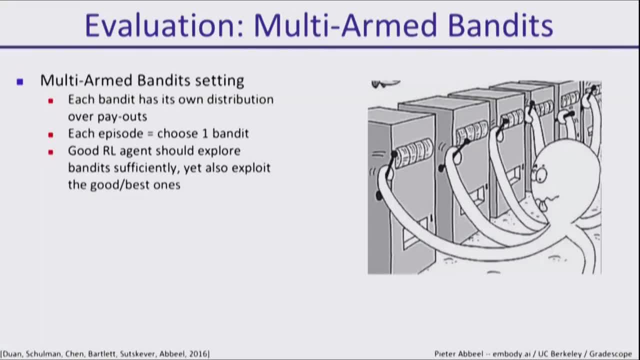 is for each of the band nets, And so you need to pull some band net arms. figure out which one's higher probability of payoff. keep pulling that one. Humans- actually expert humans- have designed asymptotically optimal algorithms for this kind of problem. 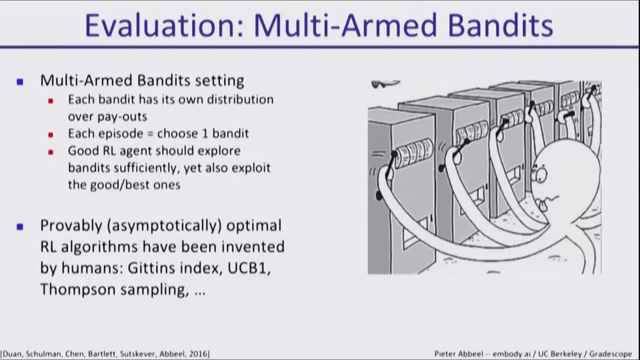 And so now we can look at: can our learned fast agent be as effective at solving a band net problem as these human-designed algorithms? So the setting here is that after training, this agent gets dropped in front of a new set of band nets it's never faced before. 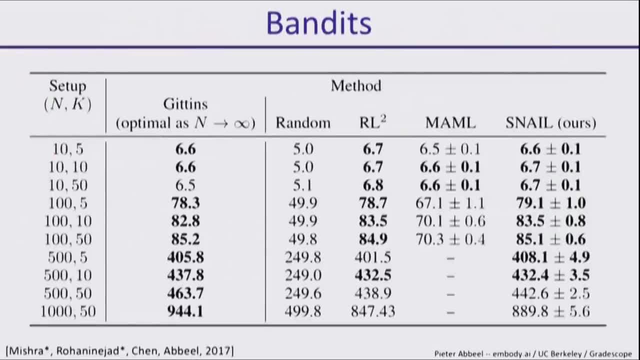 and needs to start exploring and exploiting in that new situation. Here's a table with results. The further we go down in the table, the bigger the problem setting is. What we see here is that all three approaches, some more than others, RL, squared, mammal and snail. 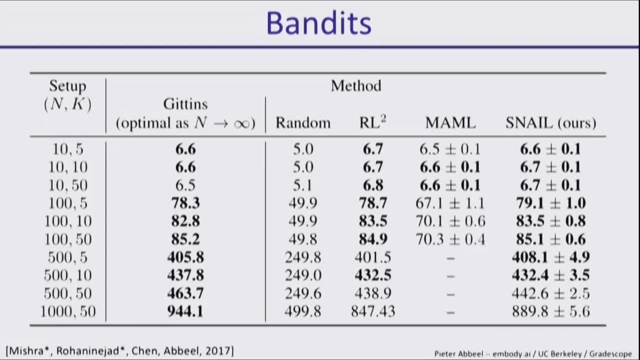 are able to be fairly competitive with human-designed, asymptotically optimal algorithms to solve this kind of problem. So this is very interesting because it means that we can learn something that's as good, or almost as good, as the best you can hope for in this kind of environment. 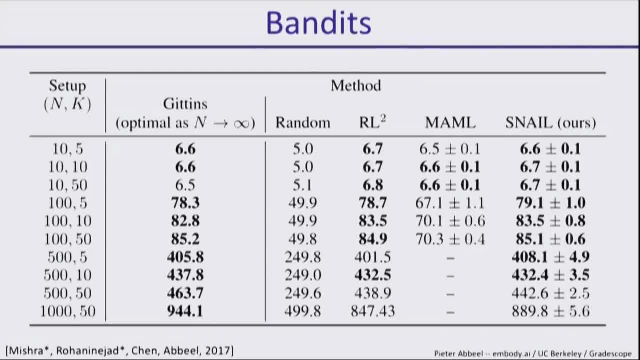 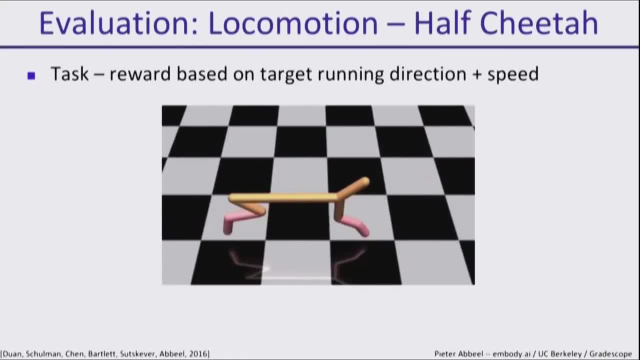 And all we need to do is run some learning. You don't need a lot of expertise into how to design band net algorithms. Here's another example. Let's say we want an agent that is really good at adapting what it needs to do when controlling. 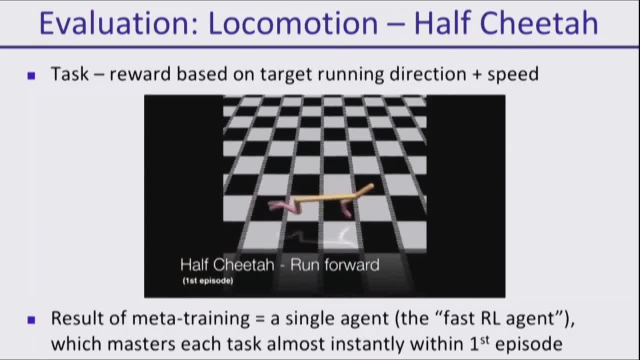 this cheetah robot. So different tasks here correspond to different speeds. So here the goal is to run forward as fast as possible. Here the goal is to run backwards as fast as possible. Now the goal is to run at zero speed, which is staying in place. 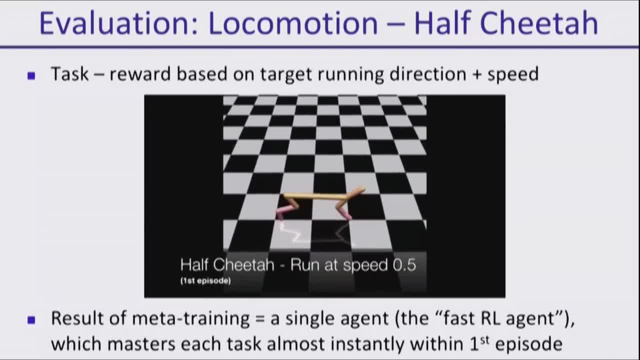 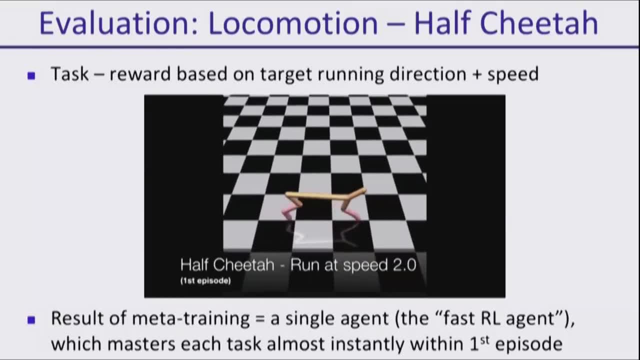 And what we're watching here is the fully trained agent, meta-trained agent being dropped in a new environment, which means a new target that it's supposed to achieve, And in the first episode- we're watching the first episode- every time adapts to what it's supposed to be doing here. 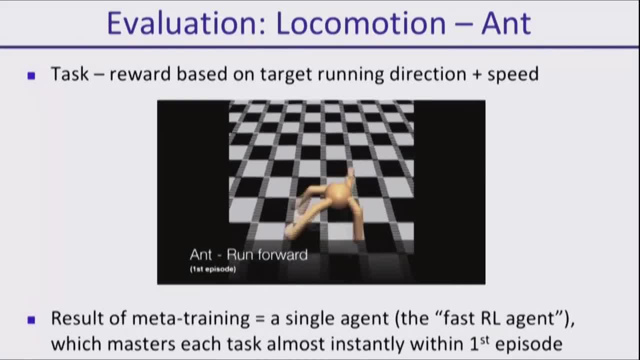 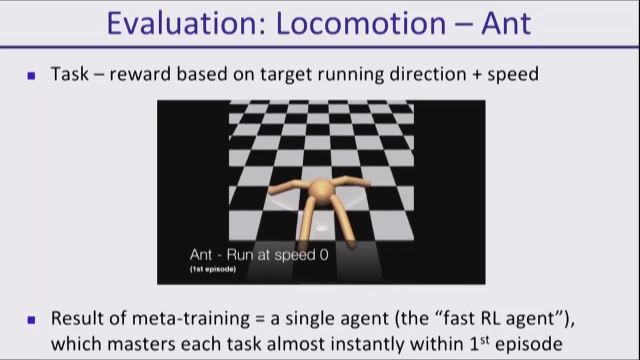 We did something similar for Antrobot. So you see, here again is the agent. You see the agent's very first episode controlling against that specific task, after in the past having meta-trained on the Antrobot and acquired a wide range of skills in the Antrobot. 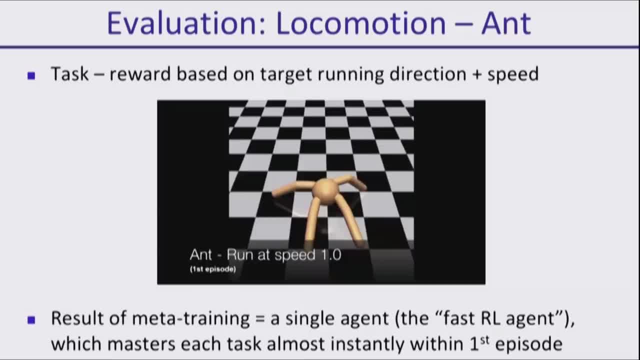 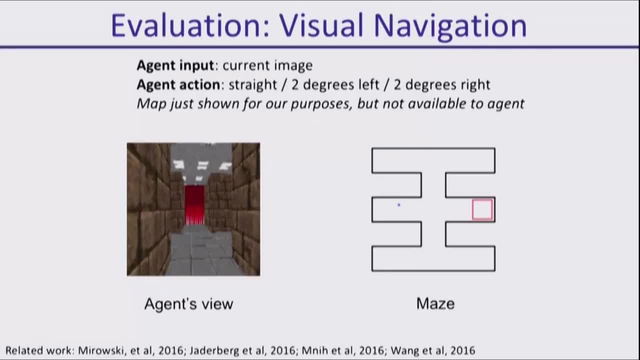 and then now getting dropped into a new environment where a new target speed is requested. Here's another example, a scenario where you need vision and control. So here an agent gets to see monocular images in front of it, gets to steer two degrees to the left, two degrees to the right, 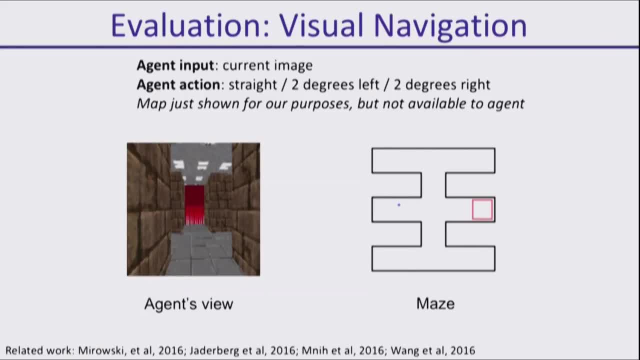 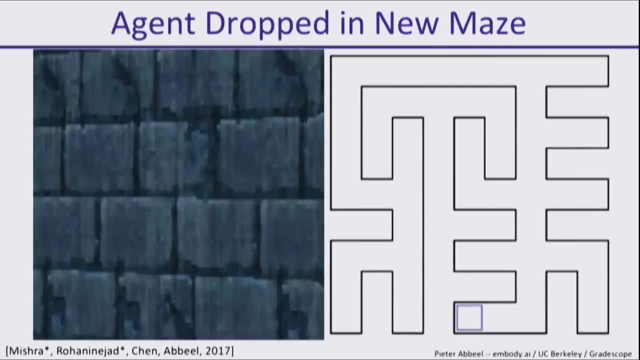 or go straight. It's supposed to navigate this maze and go to the target destination, but it doesn't have the map of the maze, It only has the monocular images, And so what we see here in action is this agent reliably navigating this maze. 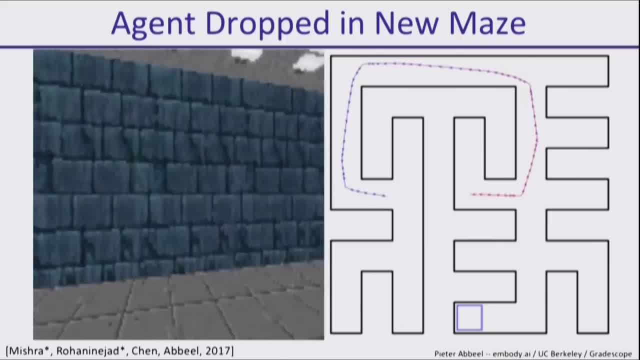 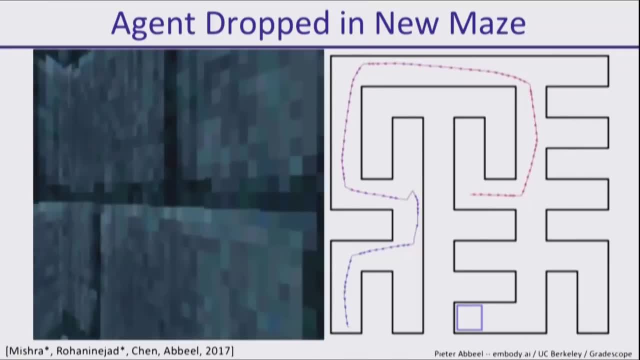 It doesn't know the map, so it's actually doing something quite reasonable. It's exploring this maze very effectively. It's never been in this maze before, but it's trained to become good at navigating mazes it's never been in before. reliably explores this maze. 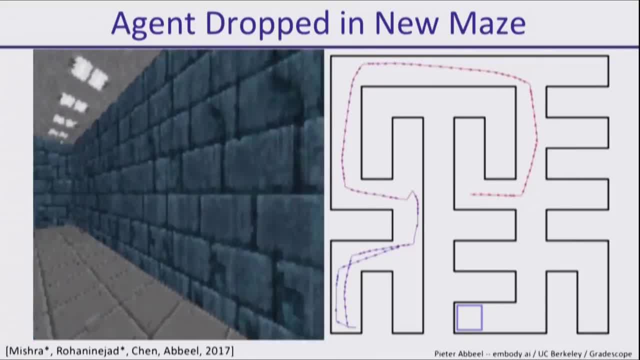 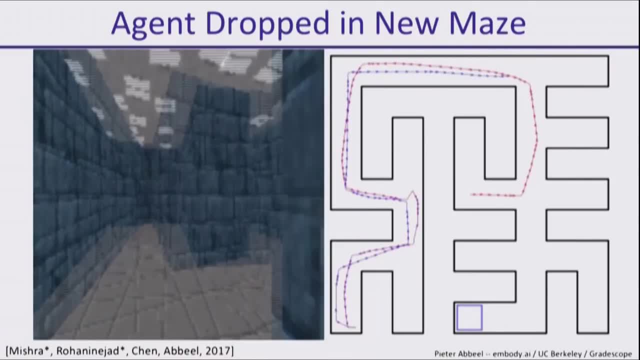 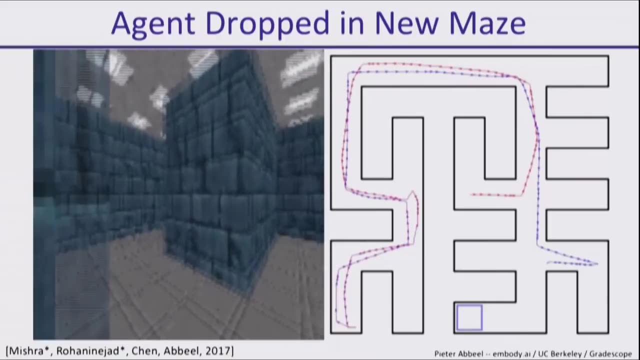 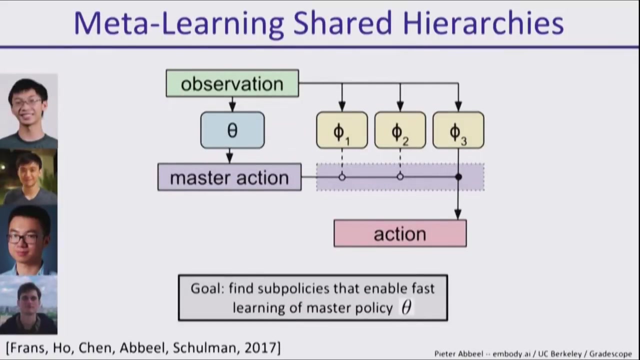 and exhaustively explores what's possible without wasting time on anything and finds its way to the other side again, Takes an unlucky turn one more time And then finds the goal. location runs right to it, So it learned a whole memory system to navigate mazes and low-level control. 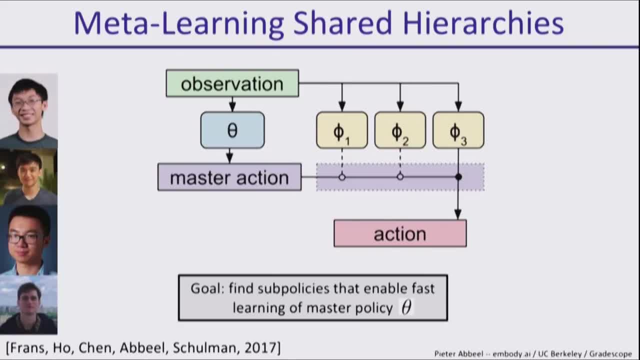 as well as low-level vision processing. If you want to do something, that is, extended actions over time, you could, for example, train an architecture like this, where you have a master policy and then sub-policies 5.1,, 5.2, 5.3, which execute at full control rate. 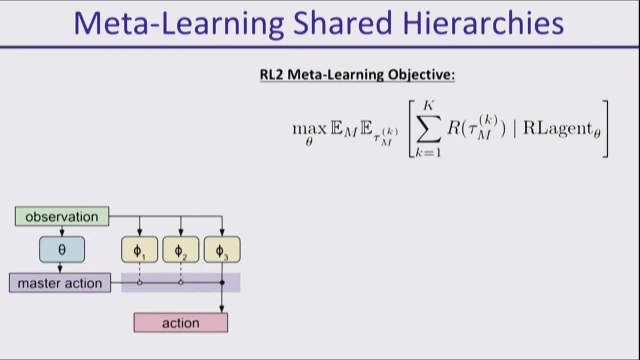 The master policy switches between them. Now you can train this in the meta-learning setting. This is the original RL squared type meta-learning setting Here. what we then do is we say: OK, let's do this, Let's find sub-policies parameterized by phi. 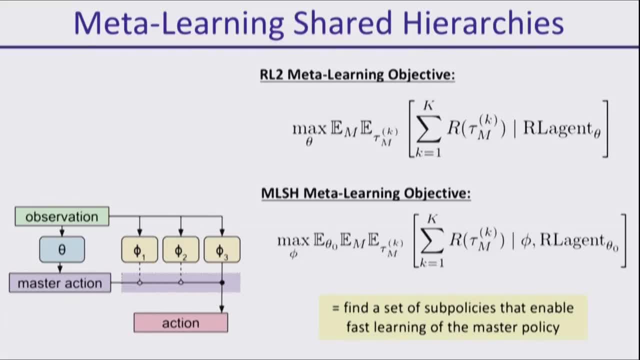 such that if a master policy is being trained by a reinforced learning algorithm and that master policy is initialized randomly with a parameter vector- theta 0, and it's randomly dropped in an environment m and gets to experience capital K trajectories, those sub-policies should. 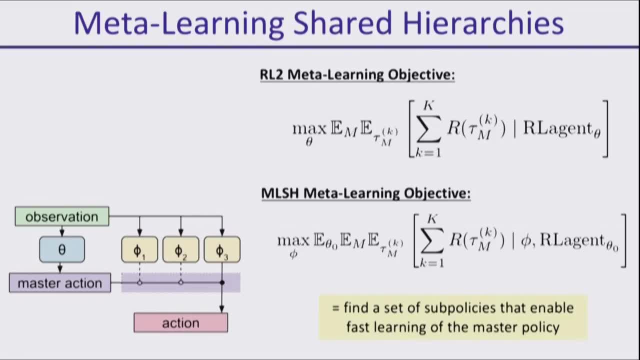 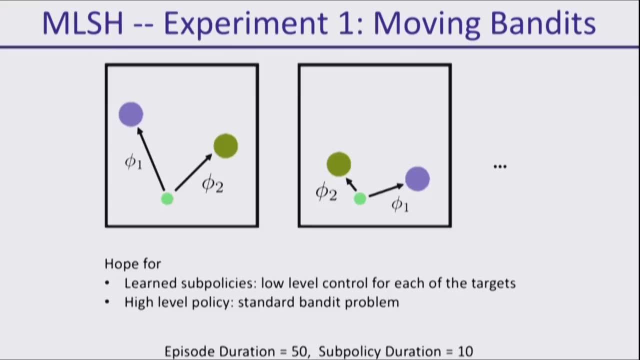 be really good at allowing this agent to succeed to train on top of those sub-policies. What you see then is that, for example, for the moving bandit problem, it learns sub-policies to go to specific, specific types of bandits. 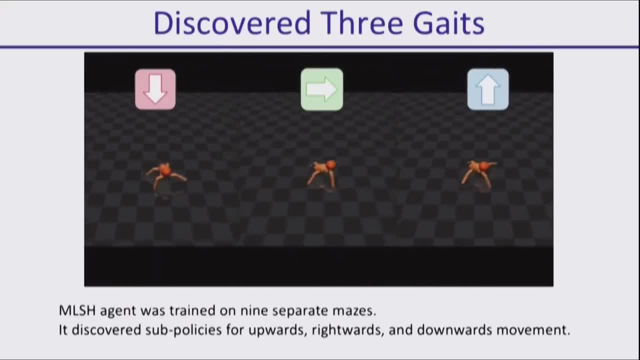 For an ant that's supposed to navigate mazes. it learns different low-level gates moving diagonally down, sideways or diagonally up, And it discovers those not by us telling that we want these gates, but by those are the gates that allow a master policy on top of this. 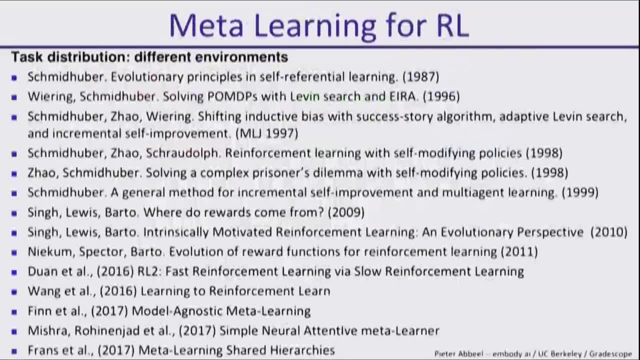 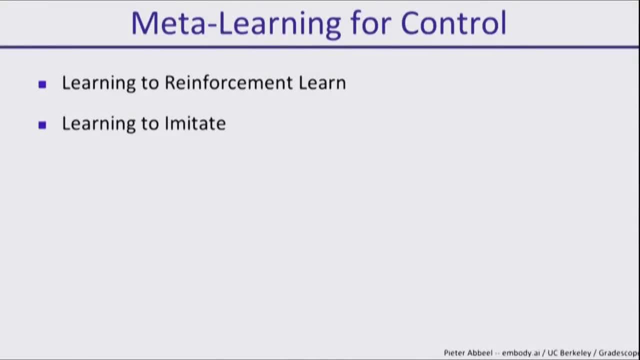 to maximally quickly adapt to new environments. Here are a few references that you can look at later. We can't just reinforce them, We can also learn to imitate. Imitation learning has been quite successful in many ways, but typically this canonical paradigm. 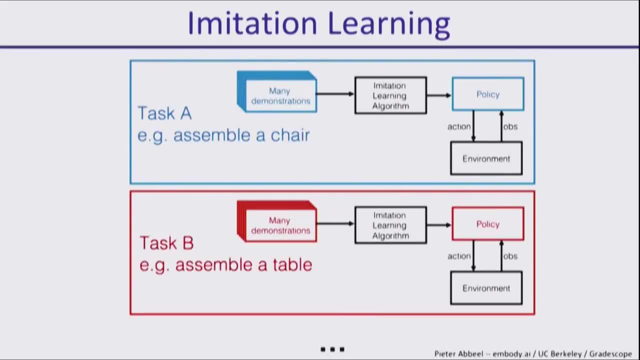 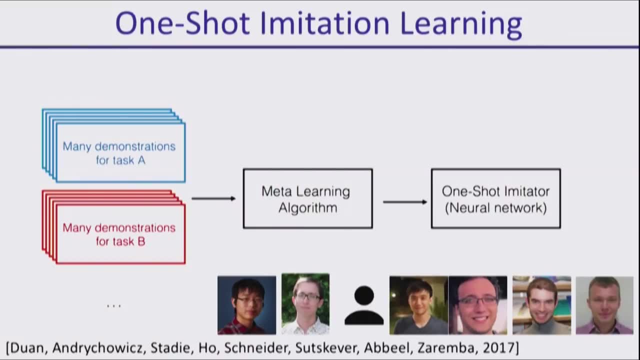 is used where you imitation learn for each task separately, So maybe assembling a chair, then assembling a table and so forth. Meta-learning would be the notion where you actually see a lot of demonstrations and then learn something that can in the future. 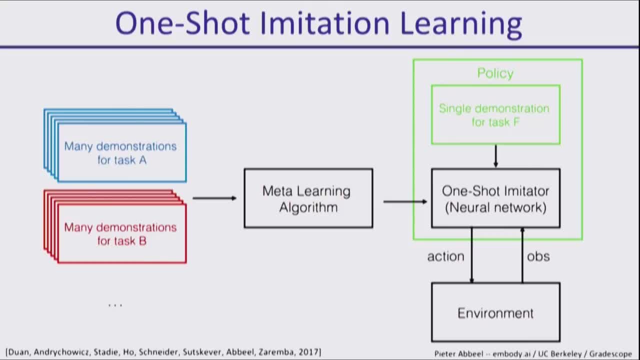 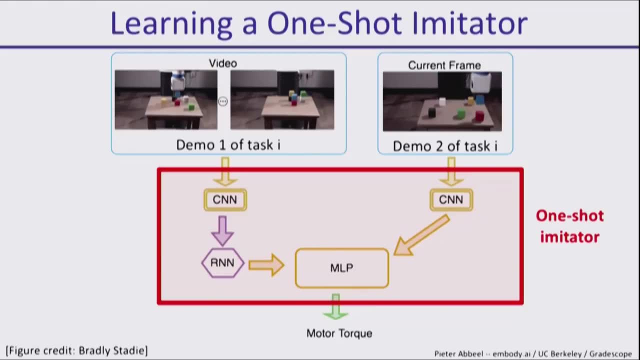 imitate from one example. So you give one example of a new task, it immediately learns how to do it. The way you can set this up is you would train a one-shot imitator- a big neural net, in this case- by showing it two demonstrations. 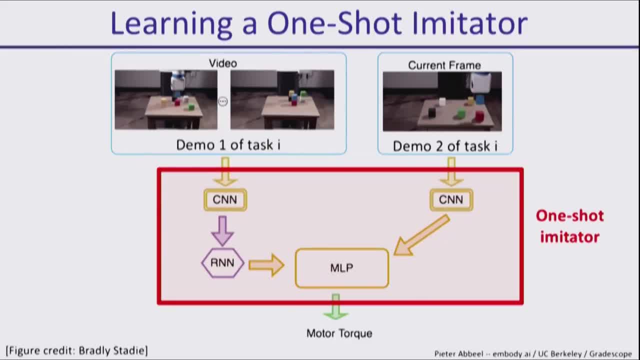 of the same task And it's supposed to, by looking at the current frame in demo two, predict what the right torque is to apply for this robot by parsing demo one. If it can do that reliably, it means that it can from that one demonstration, demo one. 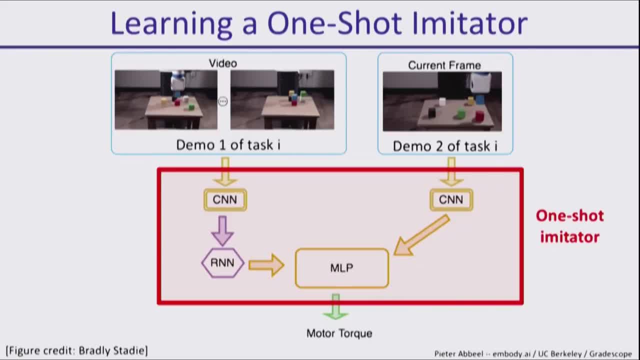 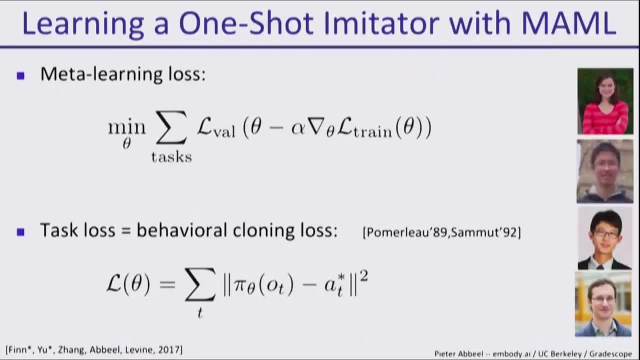 predict what needs to happen in the new situation. So this is just a supervised learning problem. the way this is set up to train a one-shot imitator. We looked at this for block stacking. I'll skip over this video. We looked at this for robot executions. 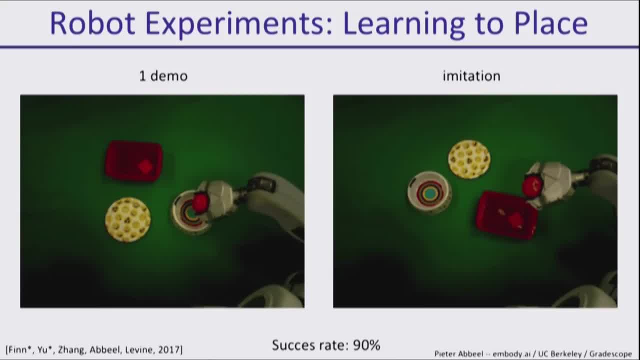 Let's watch that one. So here on the left is the demonstration The robot is placing the object into the white ball. And just from this raw stream of pixels and the torque values applied to the robot- one example- it can learn to do the right thing. 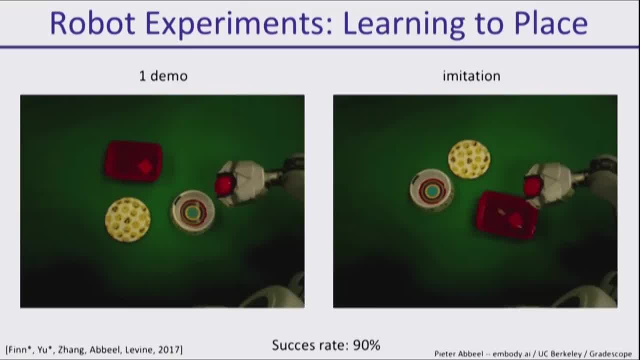 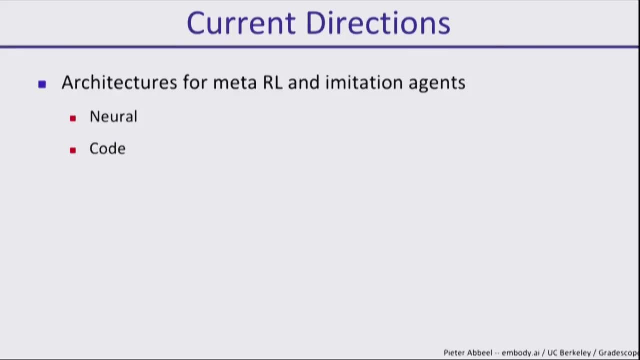 in the new situation on the right, If the demonstration puts the object onto the yellow placemat, it'll do something similar in the learned behavior, Again just from one demonstration, going from raw pixels to motor commands. OK, so what are some current directions? 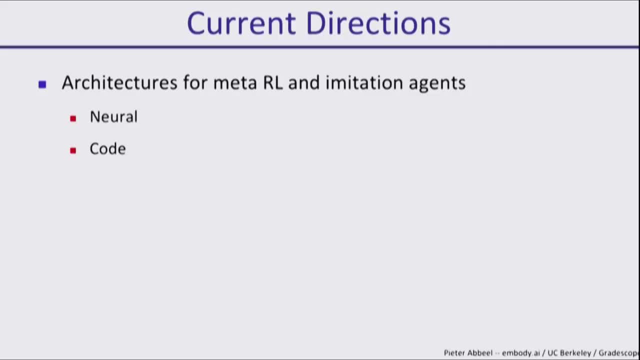 I think the examples I've shown to you are promising, but are still solving relatively simple problems compared to the real-world problems you really want to solve, And a lot more work is needed to figure out how to do that. Some of the work might be algorithmic. 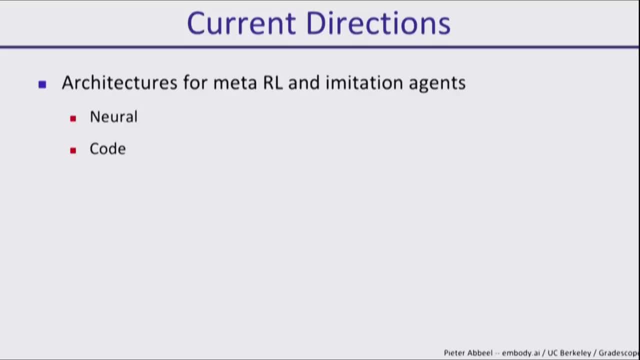 I think a lot of it will also be representationally Different neural architectures. maybe they have more memory in them than the ones I've shown here. Maybe code that is, standard programming-type representations, because those generalize really well typically to new situations. 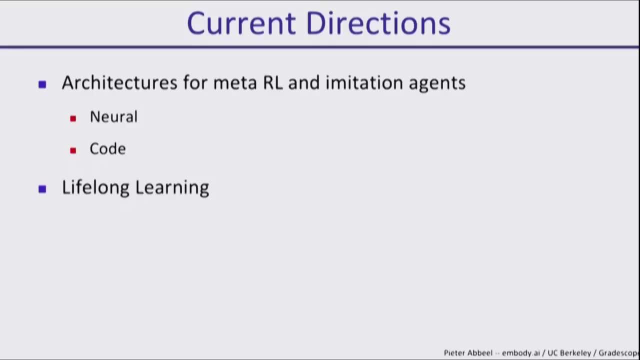 Another big challenge ahead: It's to actually move from the standard meta-learning setting. I've shown you where you get dropped in a new environment and need to do well, and then it's over to something where you continuously are faced with a changing environment. 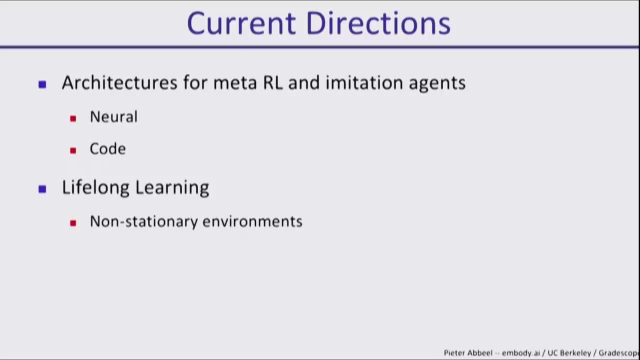 This would be the lifelong learning setting. This could be because the environment is non-stationary, or it could be because you have competition. If you have competition and the competition, the competitors are constantly adapting. you need to adapt to what they are doing or you're going to fall behind. 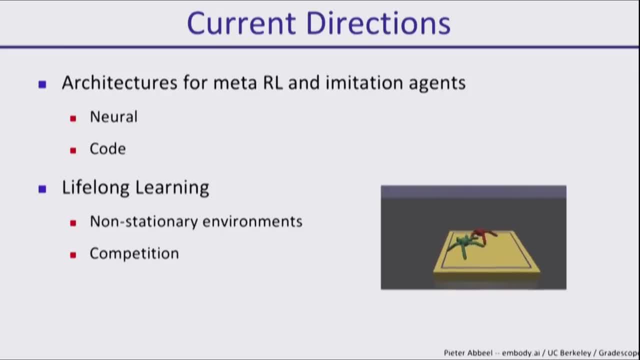 and constantly be losing. So, for example, we're watching here The red Robot. The four-legged one is a meta-learner and so is better at adapting to its opponent, And while it starts out as a weaker sumo wrestler over time. 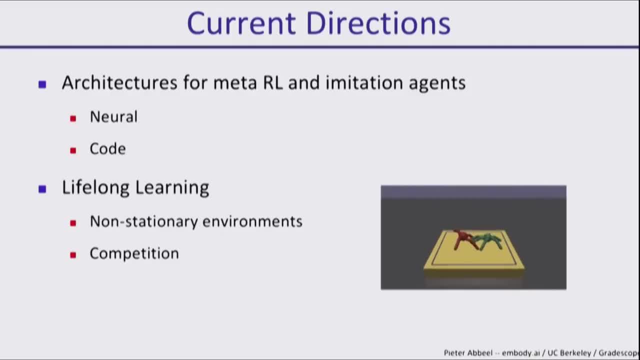 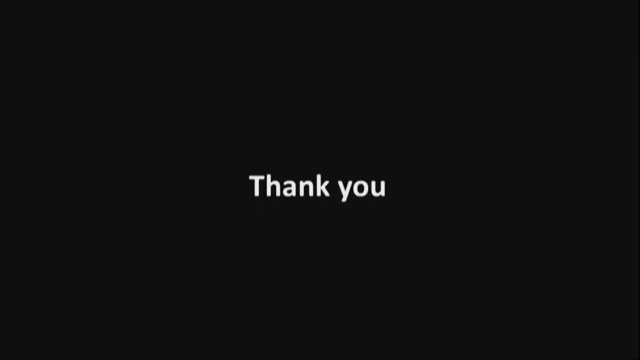 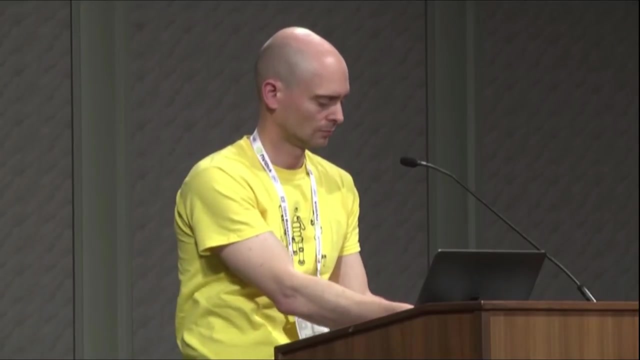 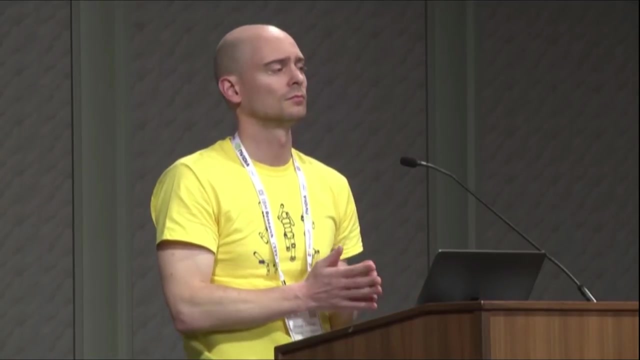 it actually starts consistently beating the green six-legged robot because that one is just using regular reinforcement learning and hence doesn't adapt nearly as quickly to changes in its environment. Thank you, Thanks. Thank you, Thanks. I have a question. I'm not sure that I understand why the metaname is very 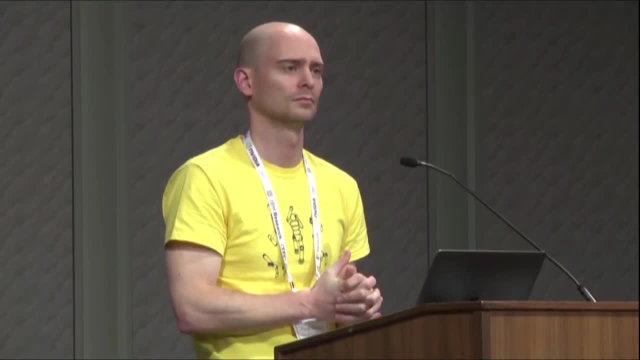 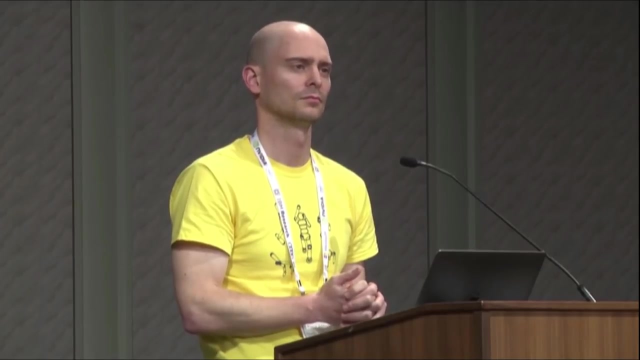 important for the reinforcement learning problem. Why it can improve the performance, since it's also based on the, I'm not sure, but I guess one of the reasons that SGD may not be enough to search in this very highly non-convex space. so the meta-learning can help the SGD, for that am I right? 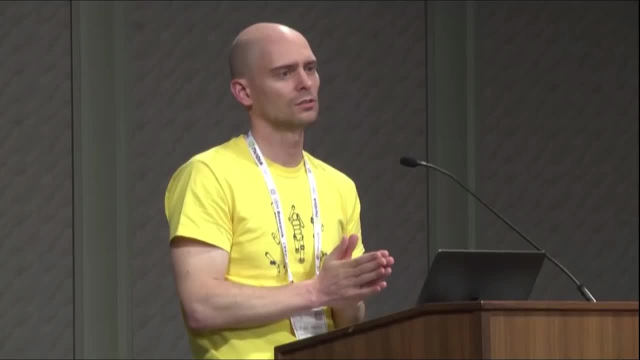 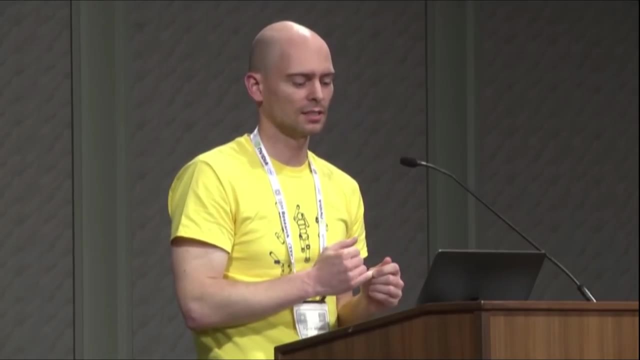 So I think there's a few parts to your question. So one part of the question is: why would meta-learning help for reinforcement learning? And so I think that's actually quite similar to why it would help for some of the other problems. And the reason it will help in reinforcement learning is because if you have a strong prior,